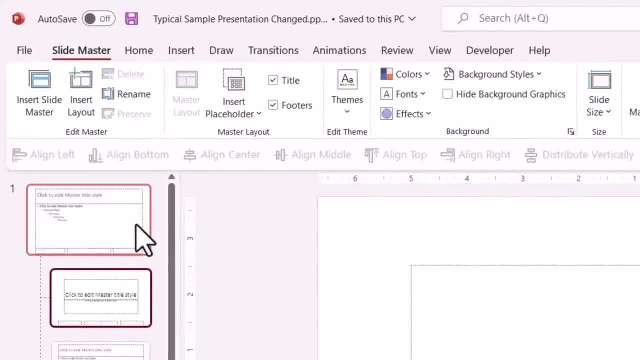 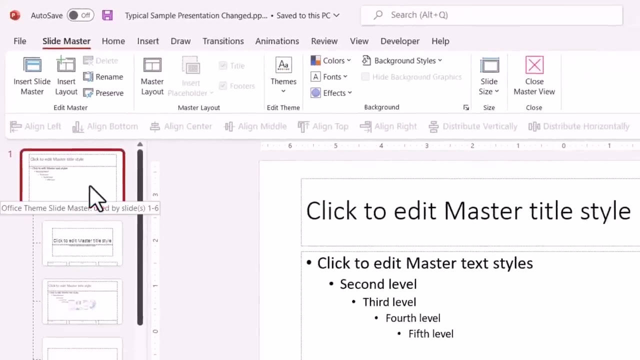 the two types of slide masters. If you move all the way up, you will see that there is this thumbnail which is slightly larger than the rest of the thumbnails, and this one is called as the theme slide master. This theme slide master influences the look and feel of the entire slide deck. 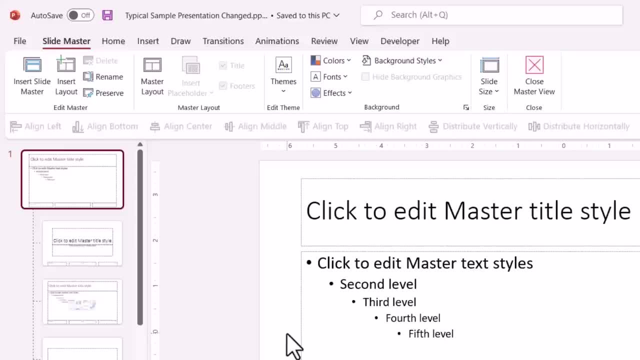 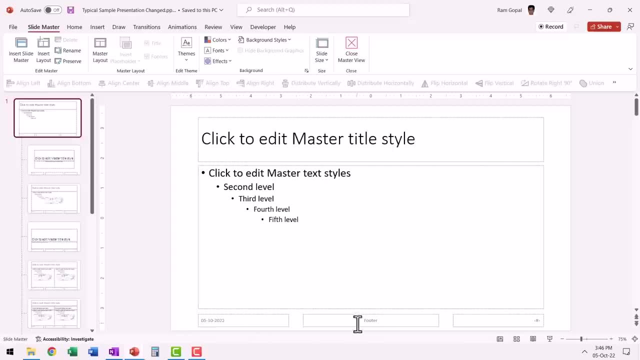 It stores all the critical information of the slide deck, like the theme used in the slide deck, the colors, the fonts, the effects, background styles, slide size and even things like the size of the placeholders and their positioning. Now, below this theme, slide master, you see all these. 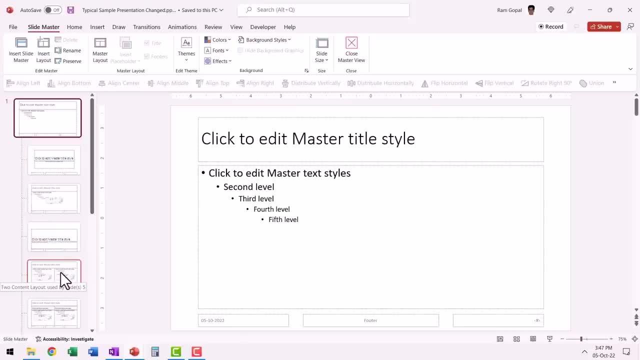 pre-formatted slide layouts. These are called master slide layouts. Now, how does this theme slide master relate to these slide layouts? This theme slide master influences all the other slide layouts, whereas the converse is not true. To understand this practically, let us do a quick demonstration Here. I am in the theme slide master. 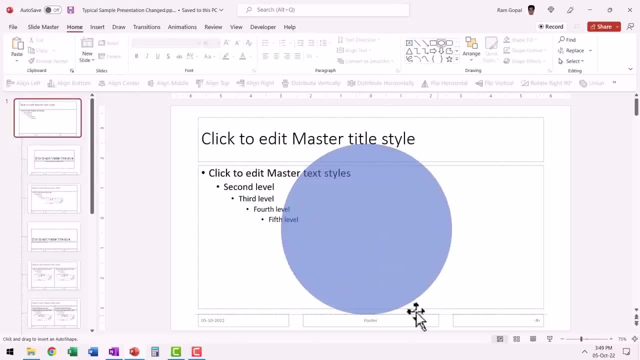 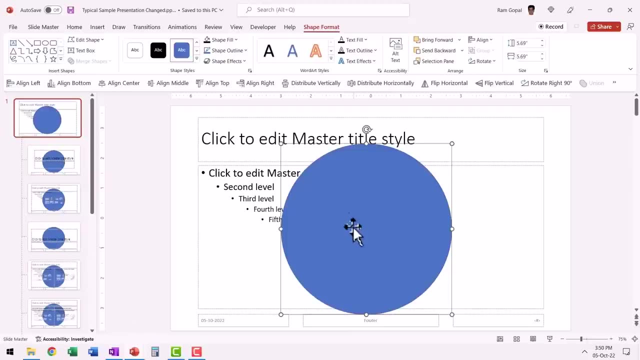 Let us go to home and let us add a large circle here. Now, as soon as I drew a circle in the theme slide master, you can see that every other slide layout has the same circle. Now let me delete this and you can see that the circle is deleted from the rest of the 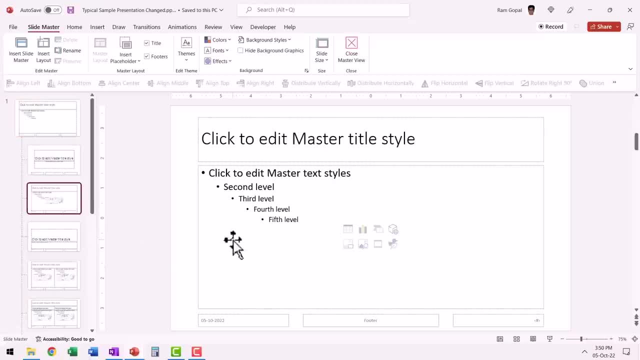 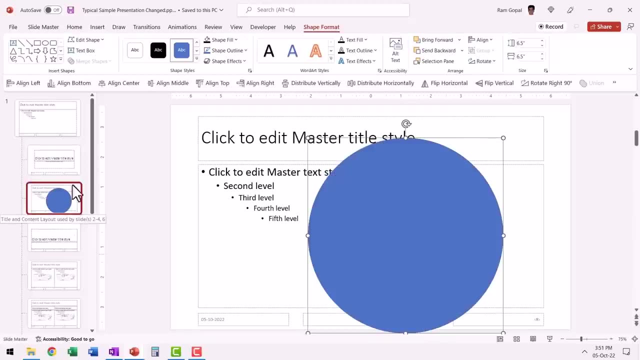 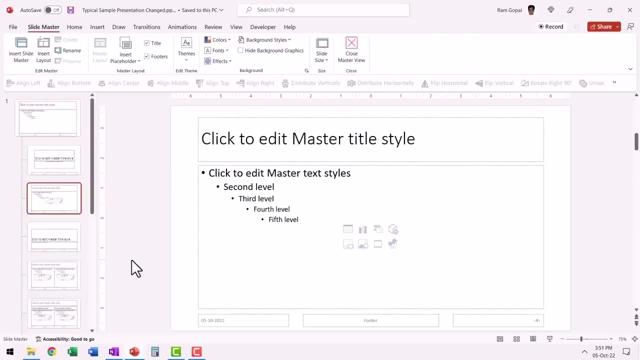 layouts. Now let me go to one of these slide layouts and let us draw the same kind of a circle here. Now you can see that the circle remains in that layout alone and the other layouts are untouched. So that is the relationship between the theme slide master and the other slide layouts. Now 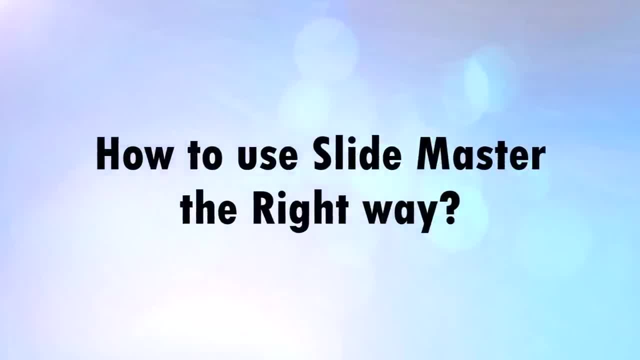 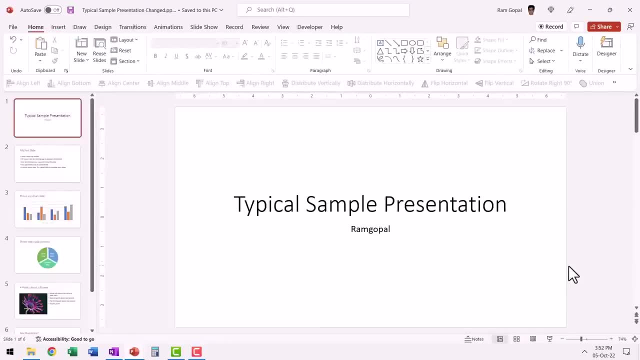 you will understand all this much more clearly when I show you a practical demonstration of how the theme slide master works. Now, for the purpose of this demonstration, I have taken a typical sample presentation. Now, when we go to the slide sorter view, you can see that these are the various. 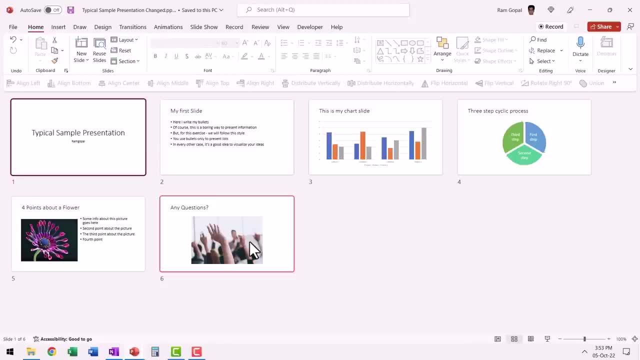 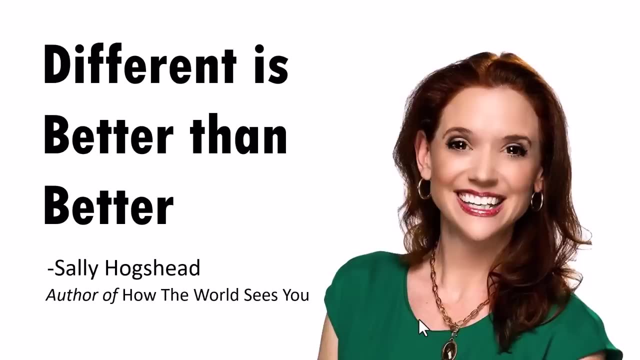 slides we have in the deck. Now we are going to improve the look and feel of this deck using slide master. First, let us score a quick win. Here is one of my all-time favorite quotes. It is said by Sally Hogshead. She said: different is better than better. This idea applies beautifully. 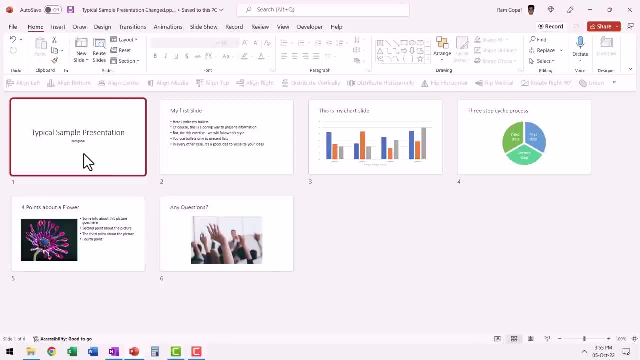 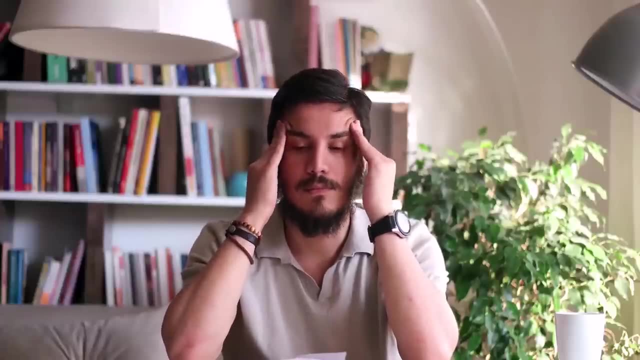 to slide design. If you want your audience to pay attention to your slide deck, then a simple trick is to make your slide deck look different from a million other slide decks your audience has already seen. So how do you make your slide deck look different? My go-to trick is to change the color. 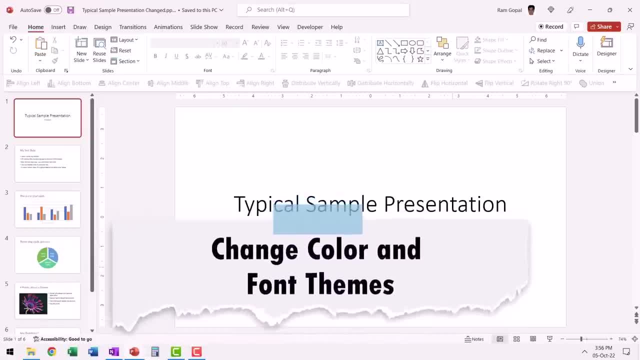 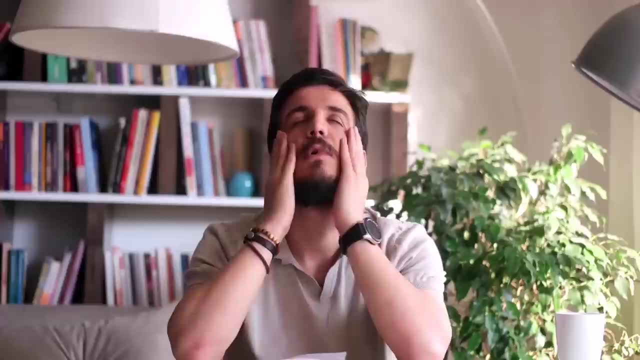 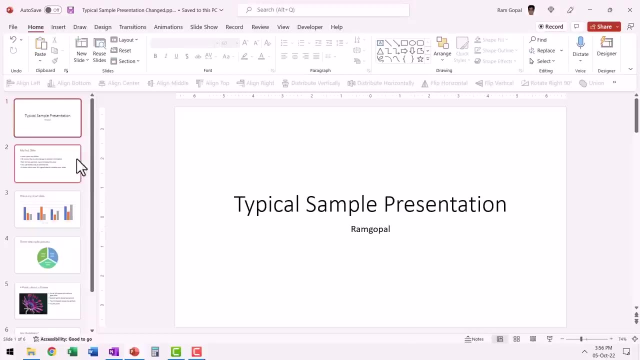 theme and font theme different from the default one. For example, you can see that this font theme, which uses Calibri for the title and body content, has been seen by your audience a million times Now. let us try and use a different font theme and see how that affects the entire slide deck. 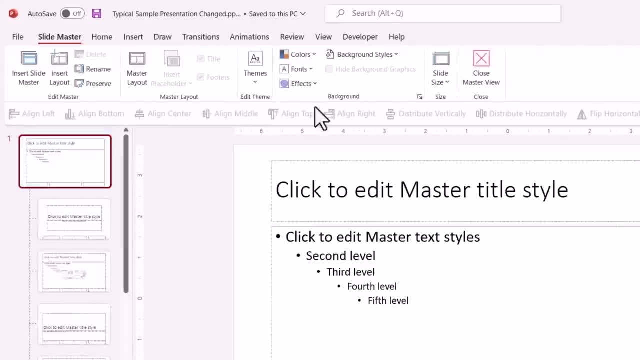 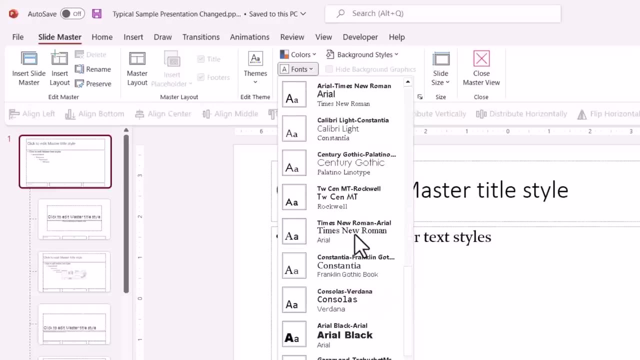 Let us go to view slide master, then go to fonts and choose a different font theme. Now let me go down, and there are quite a few beautiful options available here. These font combinations are all chosen by experts, so you can instantly make your slide deck look a lot better. 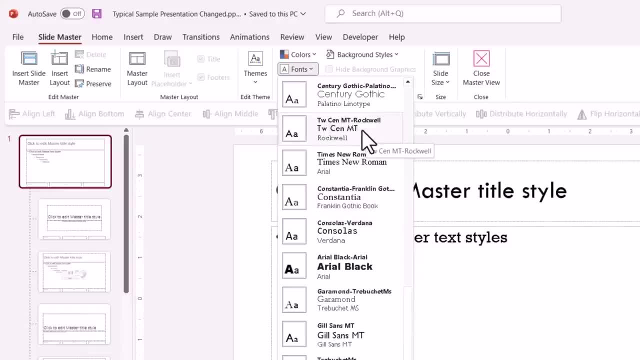 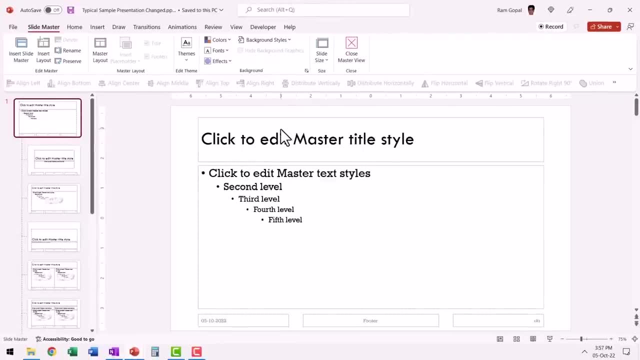 by choosing one of these ready-made font combinations. Now let me choose this one, which is Rockwell and Rockwell combination. This looks beautiful. Next, I want to change the color theme. so let us go to colors and choose a different color theme than the office one. Now let me go. 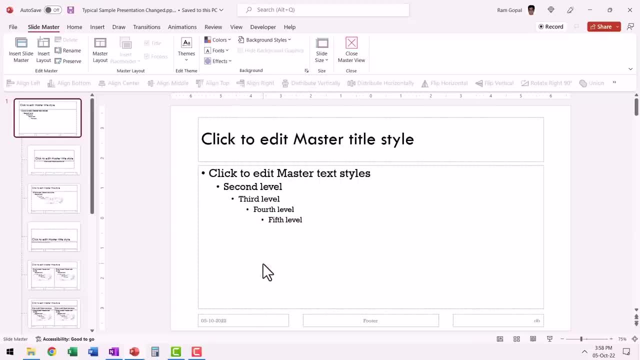 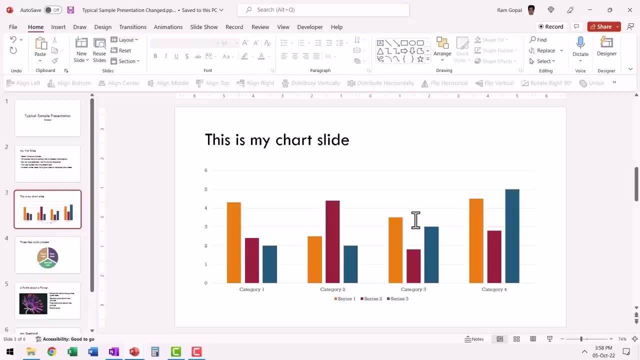 down and let me choose this one which looks very colorful, called aspect, and let me close master view. Now look at this slide deck. it looks so much better and so much more refreshing than the default look and feel. You can see that the colors used are different and eye-catching, and even the diagrams. 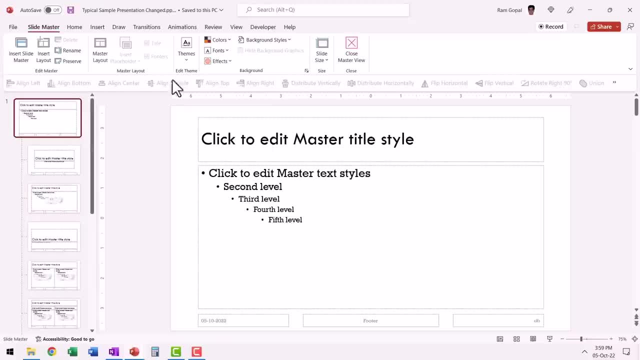 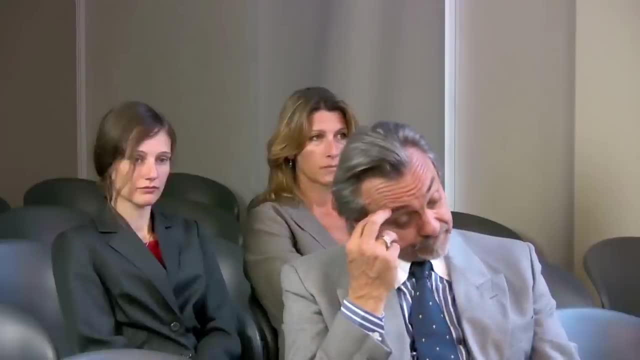 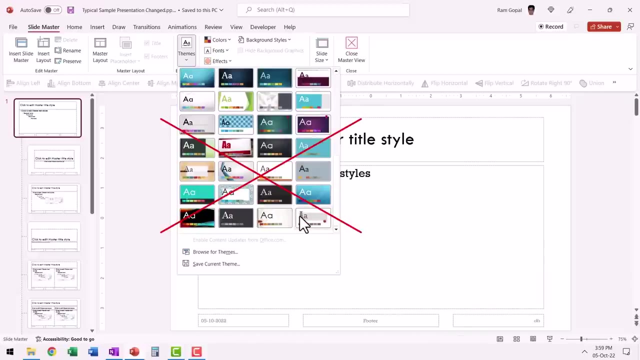 I personally don't recommend using a design theme, because the kind of design themes that are already here are used by a million other presenters, So your audience might have already grown tired of seeing these kind of designs. so it is a good idea to not choose any of these default themes. 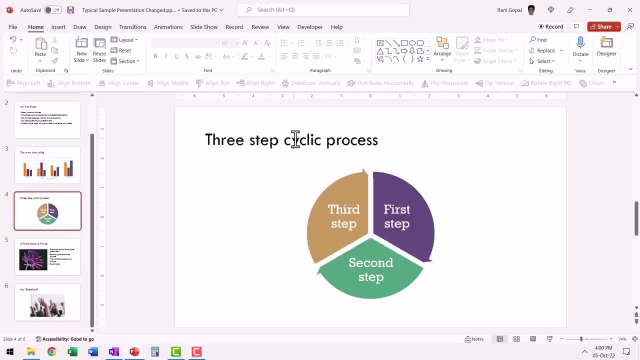 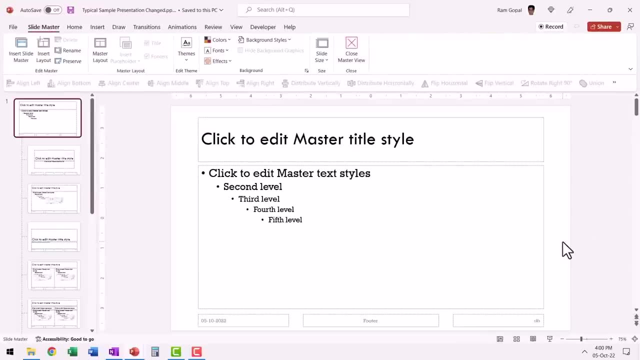 The next thing I'm going to do is to make my slide title distinct from the body content. For that, once again, let me go to theme slide master and let me make a couple of changes. The first thing I'm going to do is to draw a dark band here. so let us go to home, go to the rectangle tool and draw. 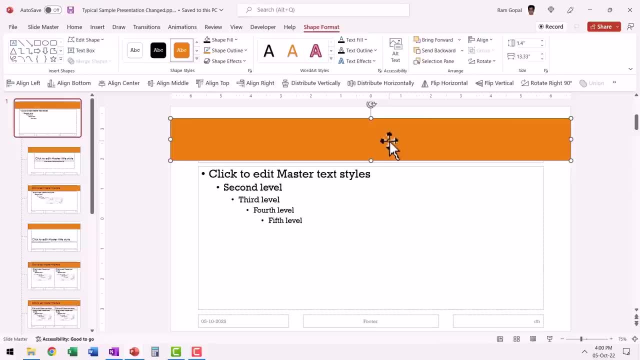 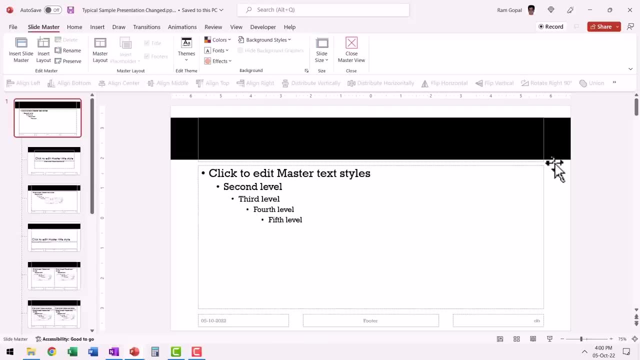 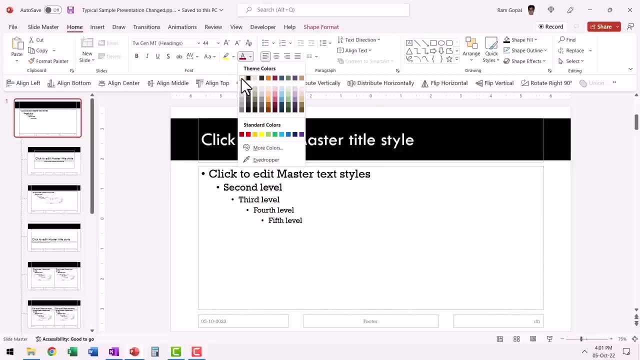 a band like so and maybe a dark color like black is a good idea. go to shape outline. say no outline. let me right click and send this to back and let us change the font color so it is easier for the audience to read what you have written here. so let us go to home and change this to. 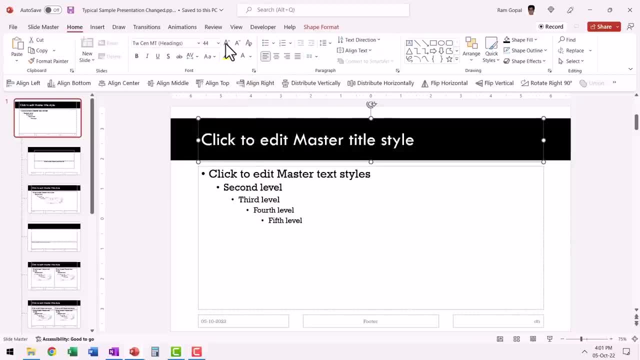 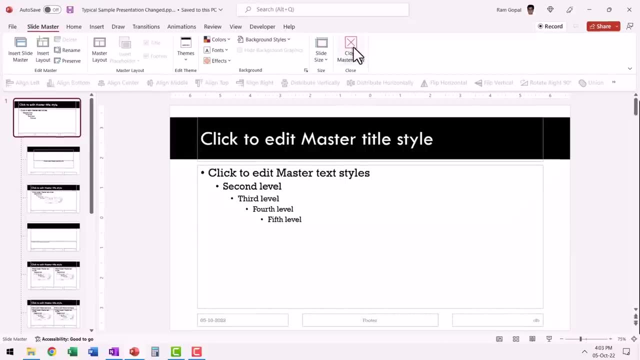 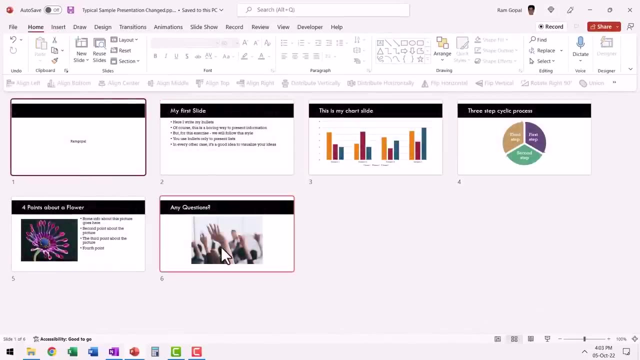 white. if I want to increase the font size, I can do so by going here and increasing the font size. now let me close master view and see how our slide deck looks. now let me go to slide sort of view. you can see that the slide design looks a lot better and more interesting. 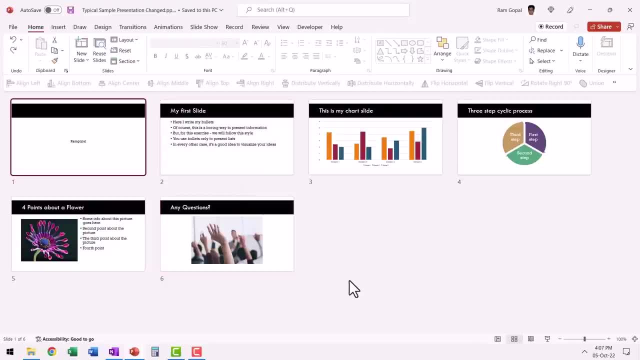 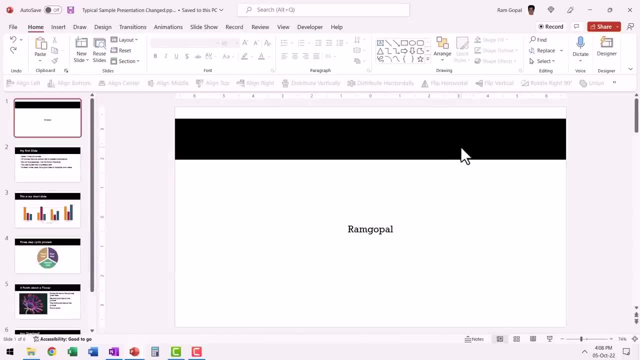 than the default look and feel that we had earlier. now I notice a couple of things in the title slide. the first one is that there is this band which appears, which I don't want in the title slide, and second, the font color seems to be white, which is not what I want. I want the default. 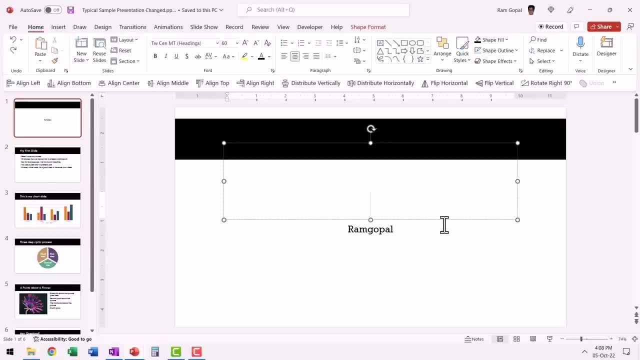 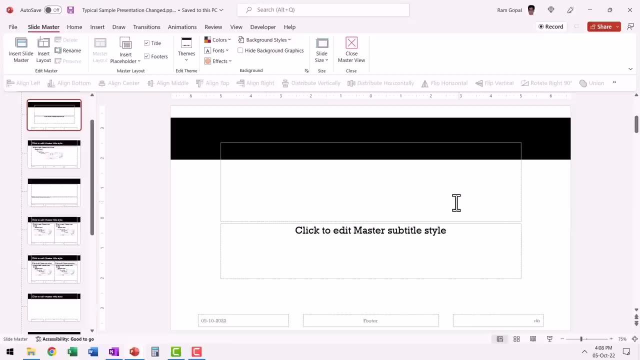 black color. so how do I make the change? very simple, let us make the change to the title layout in the master view. so let us hold the shift button down and click on the normal view. and here is the slide layout that influences the title layout design. first, let us make this visible, since we 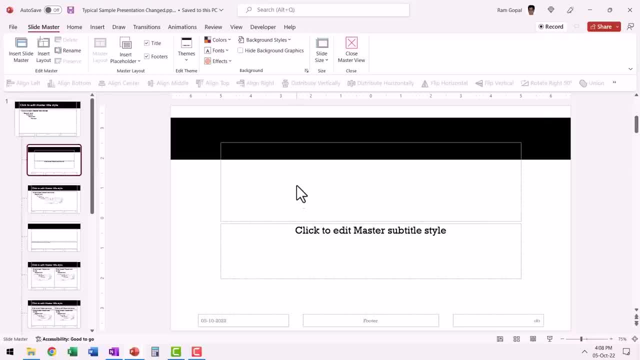 have changed the font color of the title here to white. the same thing is carried on over here and therefore, even though there is no background, the color is not visible. so let me select this and go to home and change the font color for this specific title layout. and the next thing: 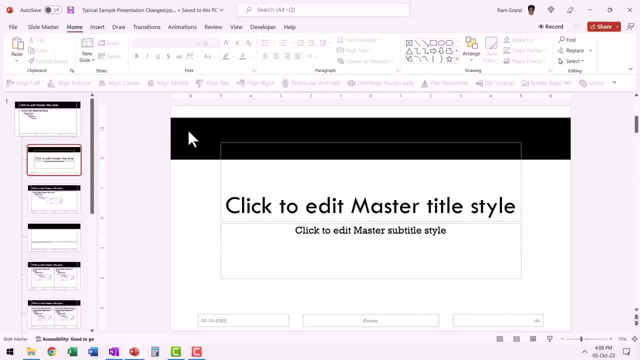 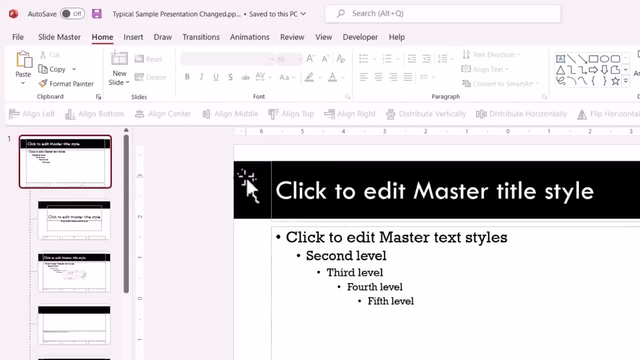 I want to do is to remove this band in the title layout. now I cannot do that because this band comes from my theme slide master and if I go to theme slide master and remove this, then the black band is removed across all the layouts. so how do I solve this issue of going to title layout and 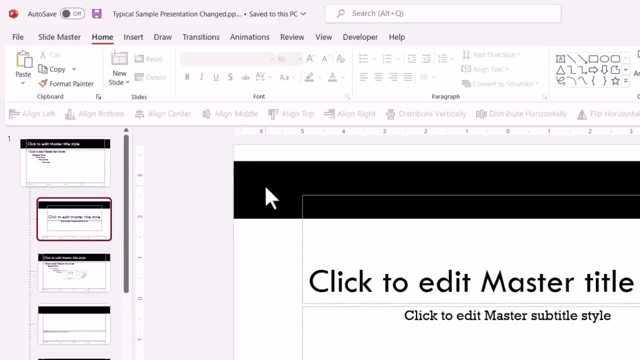 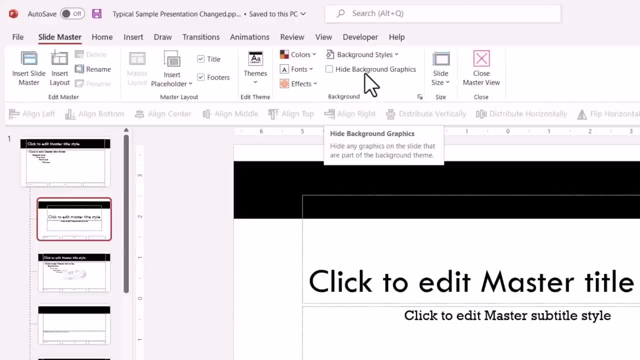 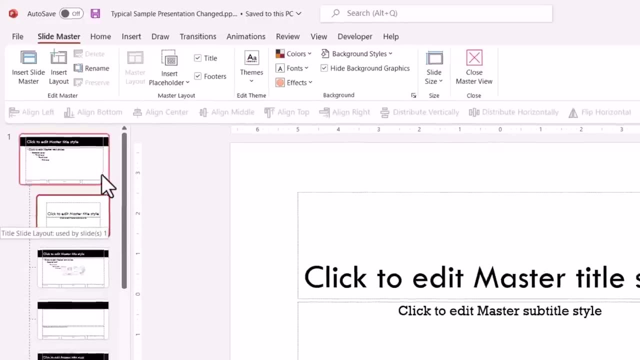 removing this specific black band. it's fairly simple. again, let us go to the slide master view, and here in the background group you see this option called hide background graphics. you check that and you see that that band is removed only for this specific layout and everything else carries that band. and we are cool. let us close master view and here we are back. 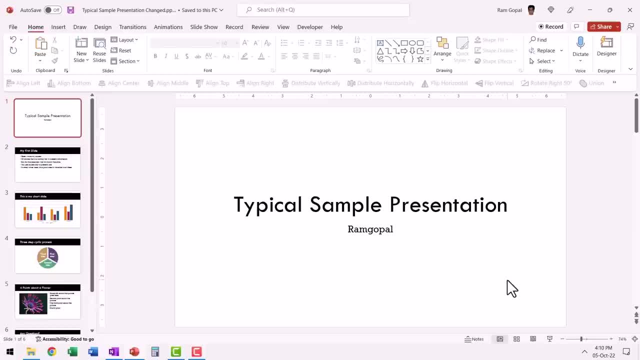 to the presentation now. as you can see, there are so many such small nuances that you need to learn about slide master to be able to use it like a pro. now the next thing we will learn is where exactly the concept of slide master come in handy in a slide design. one of the common uses is in adding: 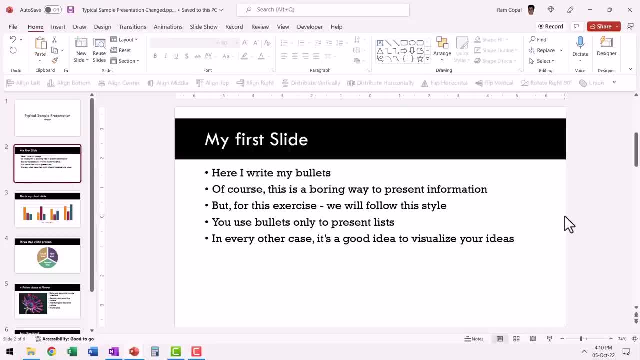 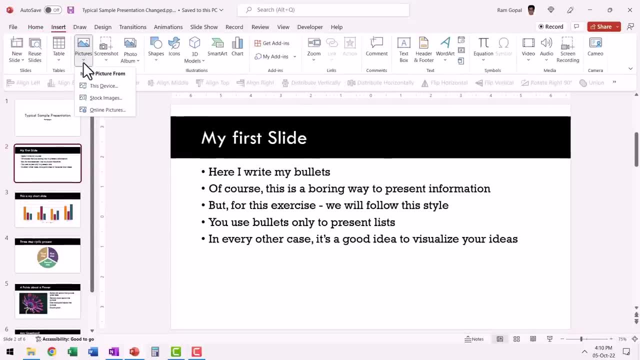 slide background. now let us say, I want to add slide background to all the slides. now what is the typical way of doing it? you go to insert, go to pictures, go to this device or wherever you have stored your textured background. let me select that here and insert. and now I have this textured. 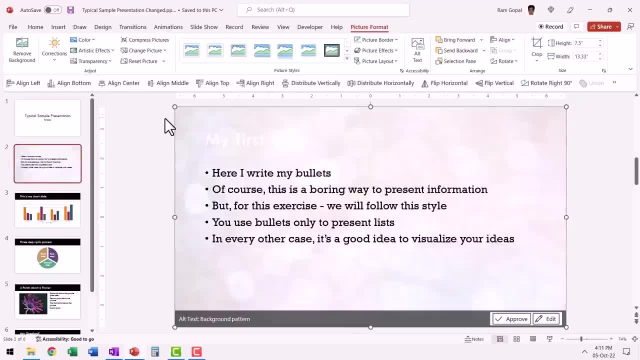 background, I can right click and send this to back now. when I do that, I can make a whole bunch of changes. now, as you can see, this is a bad idea because this messes up with our design. second, this keeps moving and, as a result, editing the slide becomes such a pain. 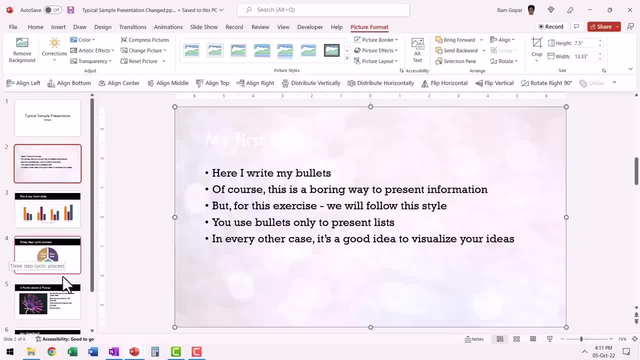 and third, if you keep doing this, by pasting this picture over and over again for all the slides, then you increase the size of the file. the reason is: let us say, this picture is 2 MB in size and your presentation has 50 slides. then by copying and pasting it over 50 times, 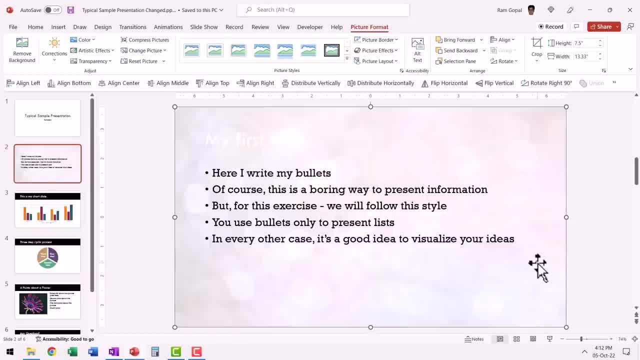 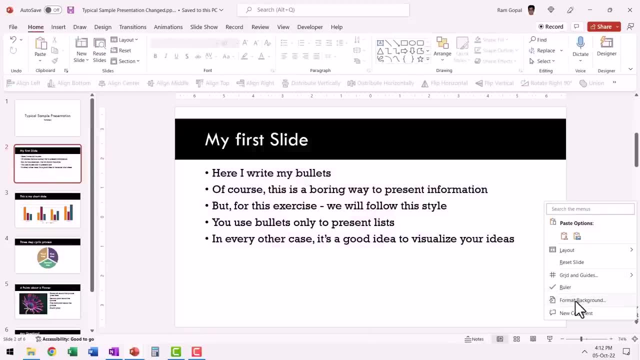 the file size to be around 100 MB, which is not a good idea. now, if you need to put this in the background, the other way is you select this ctrl x to cut it and then right click format background and go to picture or texture fill and copy it from the clipboard. this might sound like a good idea. 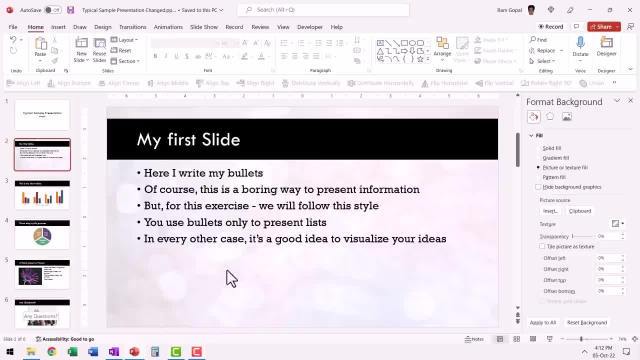 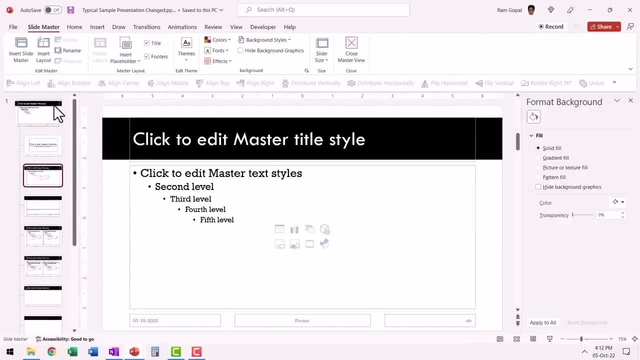 but then you need to keep repeating over every single slide, which is a pain in itself. a much better way of doing this is let us delete this and place this background in the master slide. so let me hold the shift button, click on the normal view, go to theme slide master. then go to 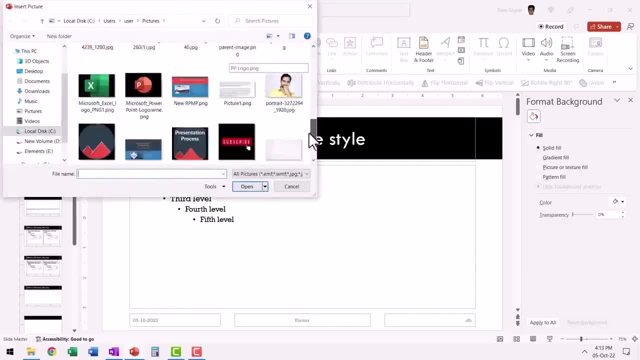 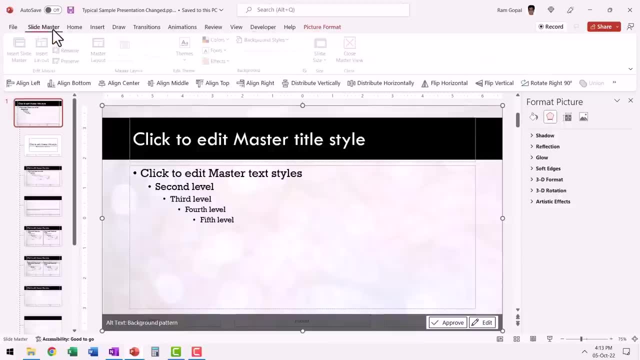 insert pictures and pick up the same image that we had used earlier, which is called textured background, and I'm going to right click and send this to back and let us go to slide master. you can see that the slide title doesn't really have that and that is because we have hidden the background. 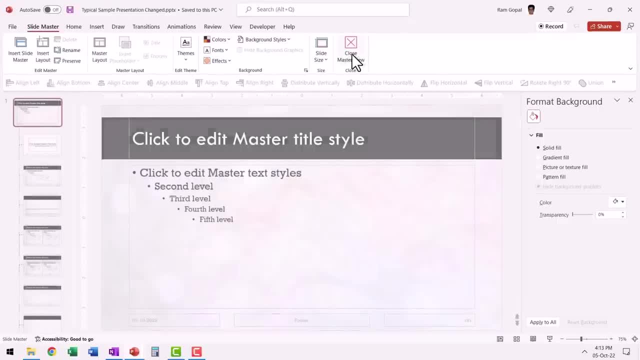 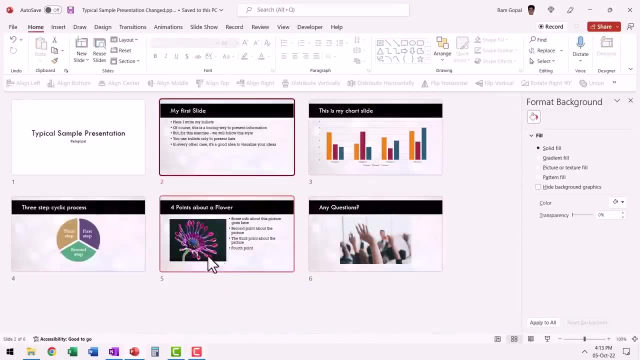 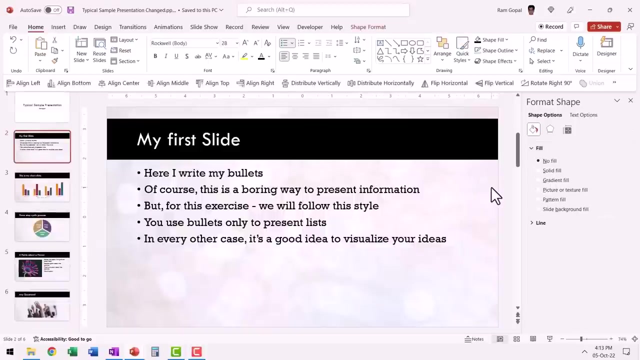 graphics here, so it works pretty beautifully for us. let us close master view and here you can see slide has the same background. now the presentation is not going to be so heavy because the pictures are not pasted over and over and again. when i go to the slide, you can see that that picture 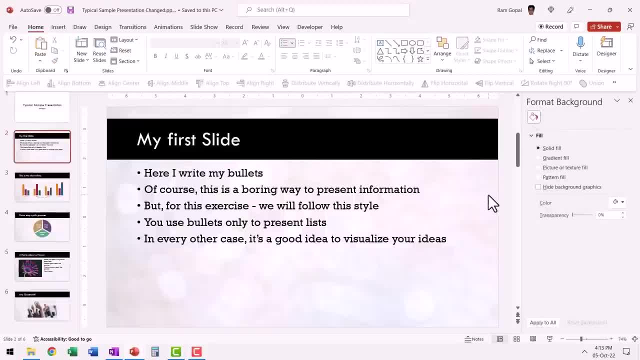 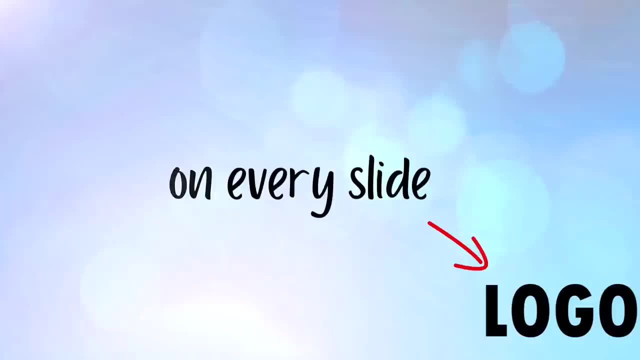 is in the background, so it doesn't affect my slide editing capabilities. another common reason why slide masters are used is to place a logo on every slide of your presentation, though i personally wouldn't recommend placing a logo on every slide because it doesn't really serve much. 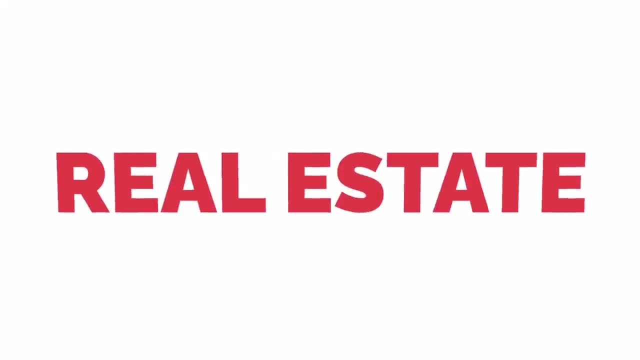 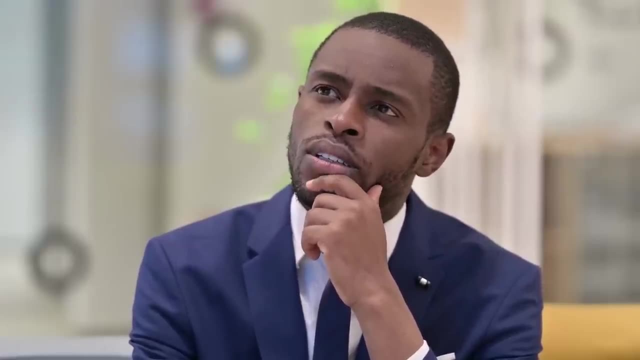 of a purpose and it actually wastes precious slide real estate. there are certain people who would want to do it. in such a case, i want to show you how to place your logo on every slide, but in a non-intrusive way, that is, by placing a washed out watermark version of it. let me show. 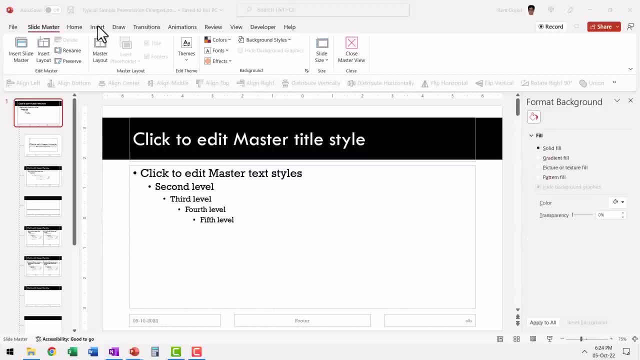 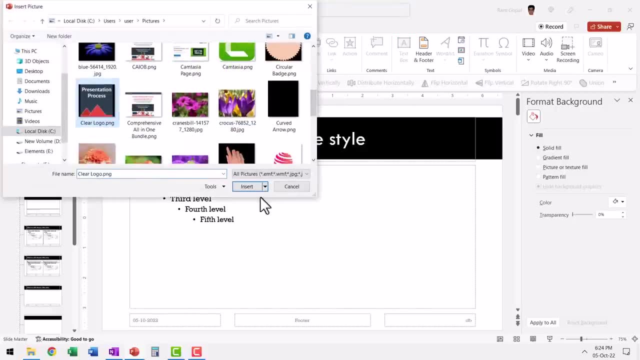 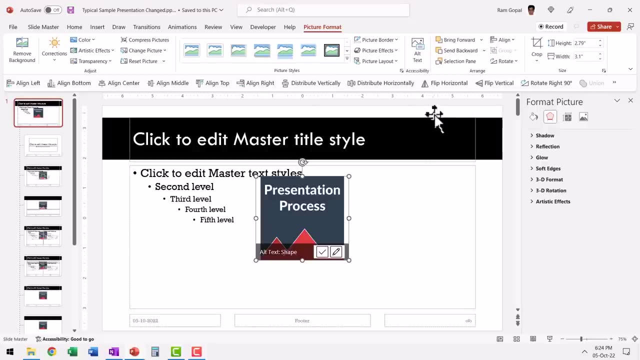 you how it is done. here we are on the theme slide master. let us go to insert. go to pictures. go to this device. i have stored my company logo, which is presentation process. let us insert that. you can see that the color scheme of my logo is very different from the color scheme that is used on. 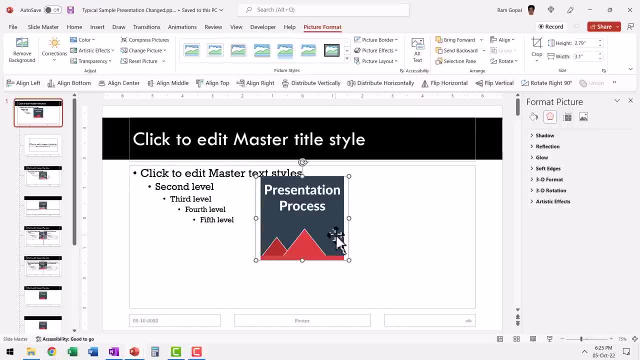 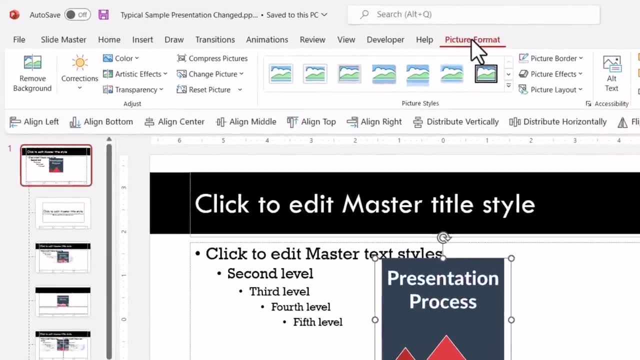 the slide. so by placing this i actually would disturb the look and feel of the slide. so let me reduce the intensity of these colors by selecting this image, and we're going to picture format color, and let us choose in the recolor option, this option called wash out. now you can see. 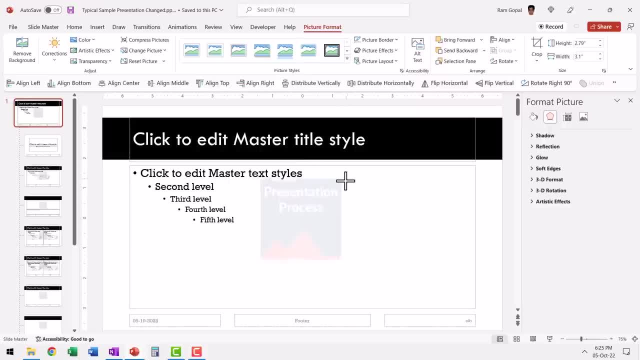 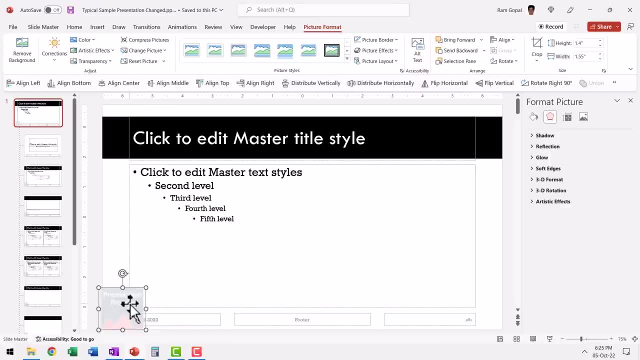 that the logo is washed out. now i can reduce the size of it and i can place this somewhere in the bottom left corner or wherever you want to keep it. now. here, i have increased the size so you can actually see. now let us go to slide, master, and. 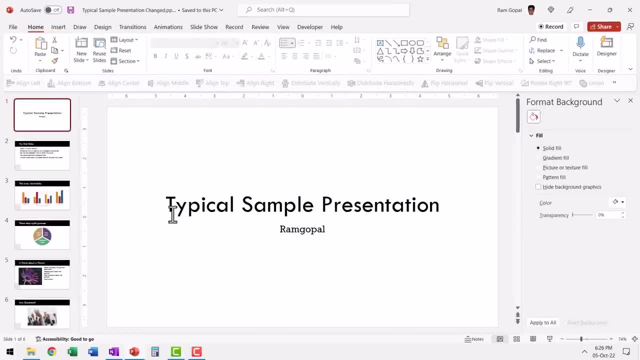 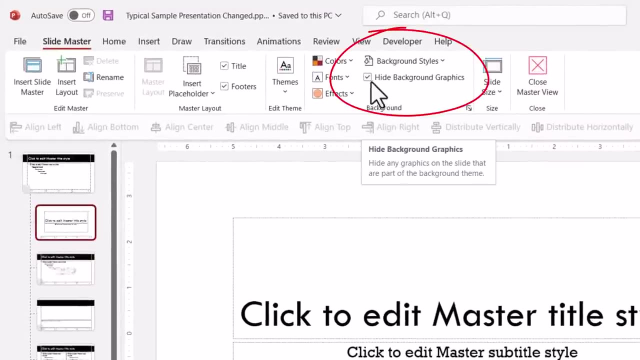 close the master view now on every slide, but for the title slide you can see that the logo is placed. why is it that we don't have a logo on our title slide? when we go to view slide master and when we go to this title layout, you would notice that there is this option. we have checked earlier. 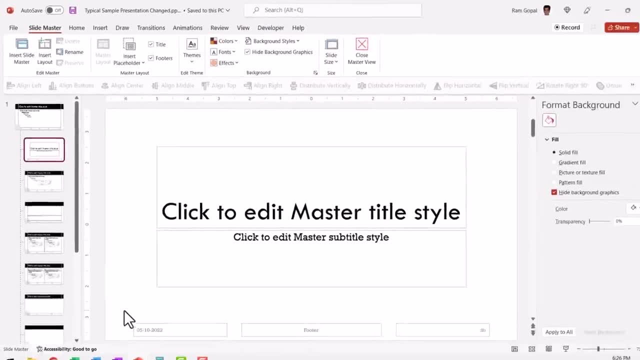 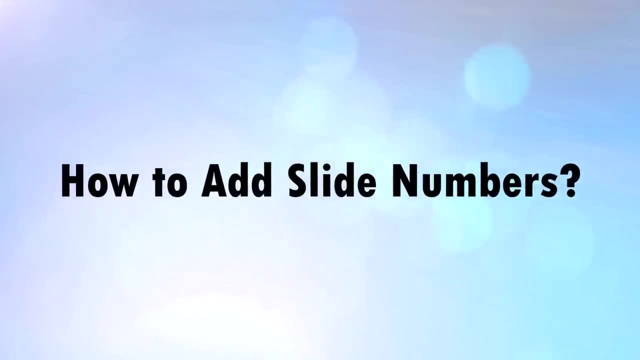 called hide background graphics, and that is the background graphics that we have selected here. so is the reason why that logo doesn't appear on the slide title. let us close this. next, let us learn how to insert slide numbers on every slide, for that first you need to go to insert, then in the 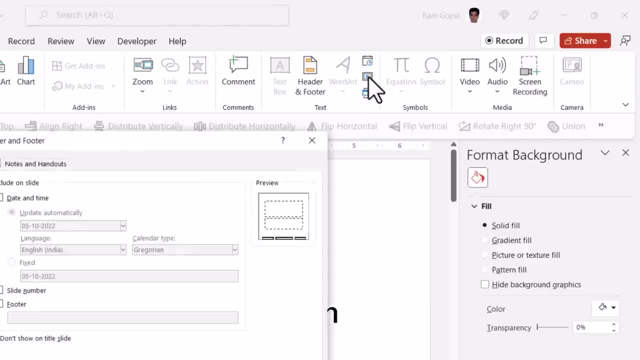 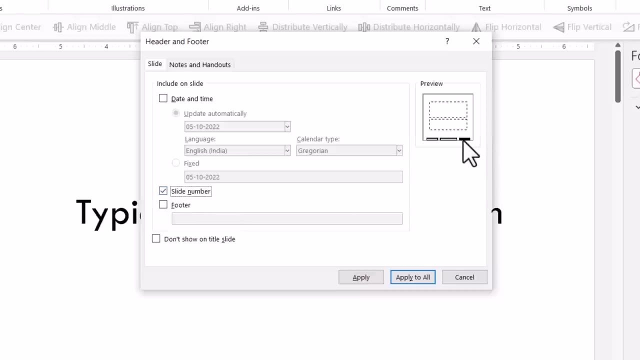 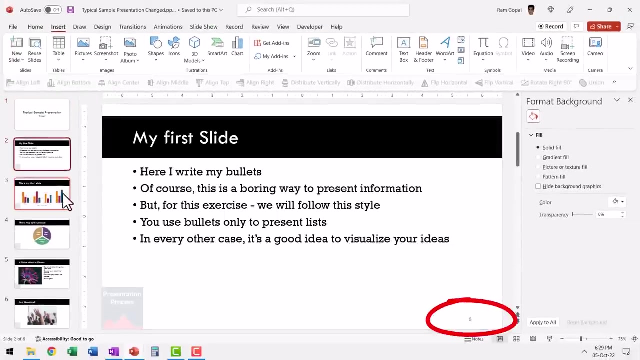 text group, go to this option called insert slide number. you get this dialog box in that you check the option called slide number and that shows you where exactly the slide number will be shown and you say apply to all. now the slide numbers will be available on every single. 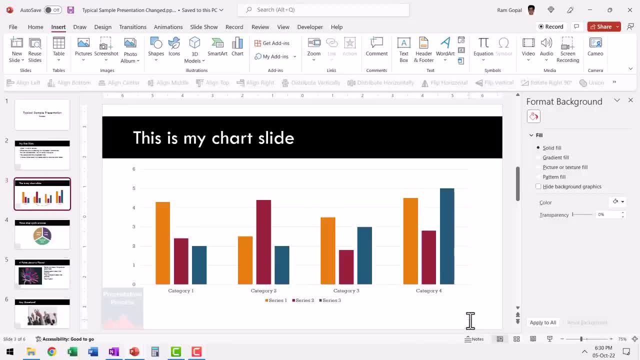 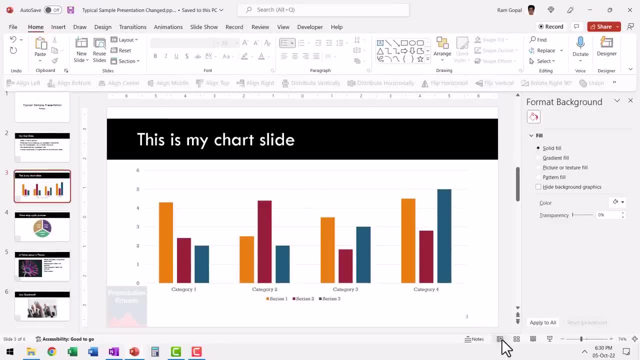 slide, as you can see here on the bottom right corner. now to change the font color, font size, font type, etc. you need to go to theme slide master. so let us hold the shift button down, click on the normal view, then go all the way up to theme slide master. now here is the place where you make all. 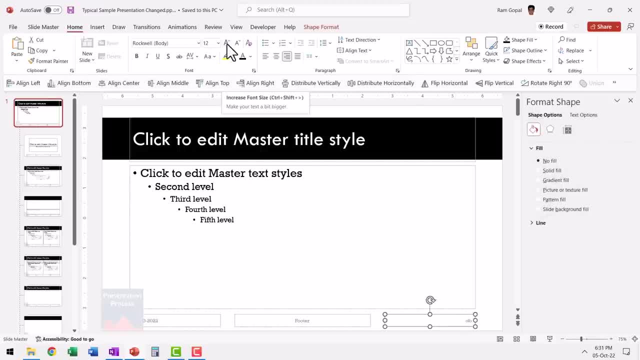 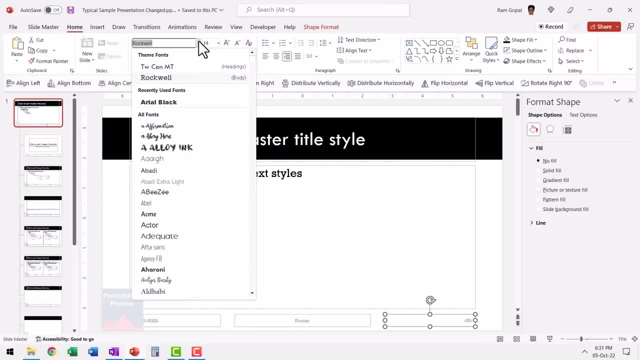 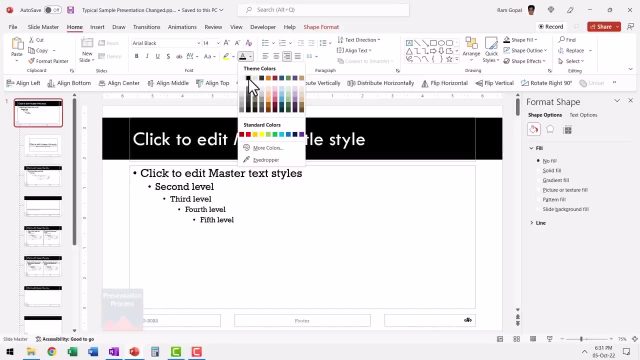 the changes. if you want to increase the font size, you can do so by going to the home tab and by increasing the font size, like this. if you want to change the font type, you can do so like, say, i want now let us make this slightly darker by going to the font color and choosing black color for. 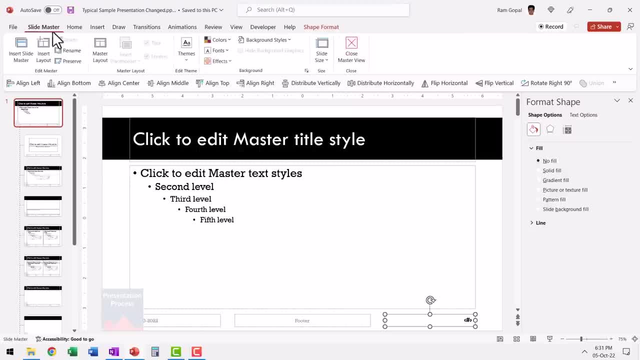 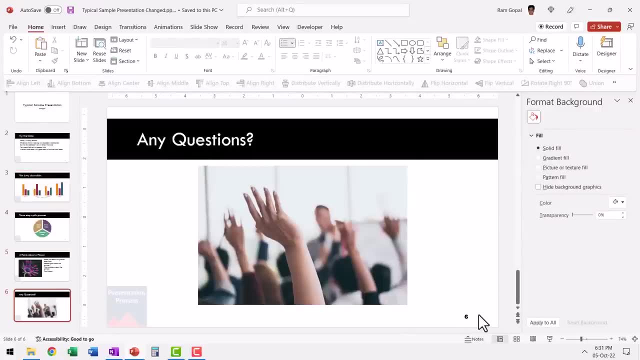 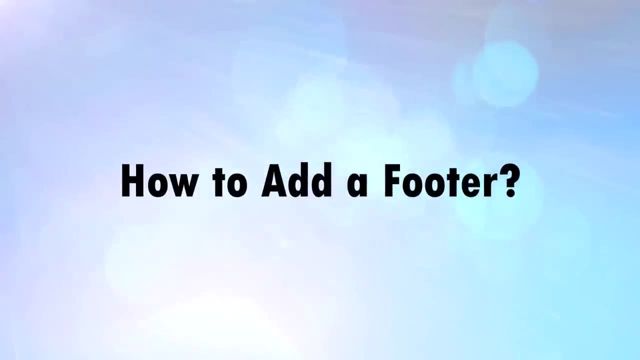 this, so it is clearly visible. let us then close the slide master view. so let us go here and say: close master view. now you can see on every single slide the slide number is clearly visible, just as we added slide numbers. if you want to add a footer for some legal disclaimer, on every single slide, as 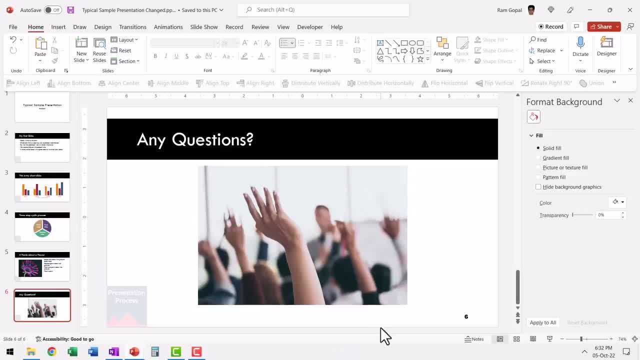 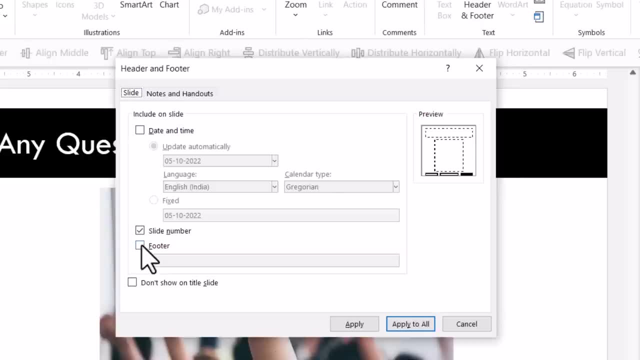 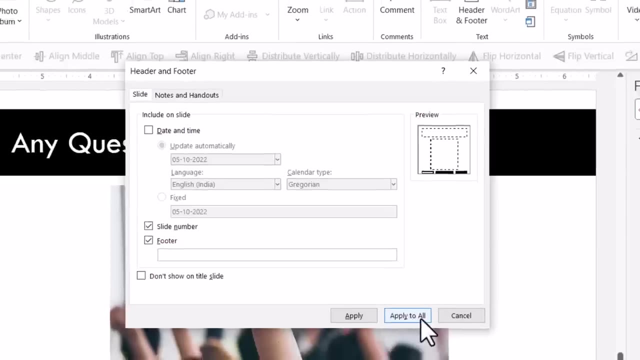 it is mandated for some of the finance presentations or legal presentations, you once again go to insert, then go to the same insert slide number option and here you check the option called footer and you write your text here and the job will be done and once it is done you say apply to all. so that is. 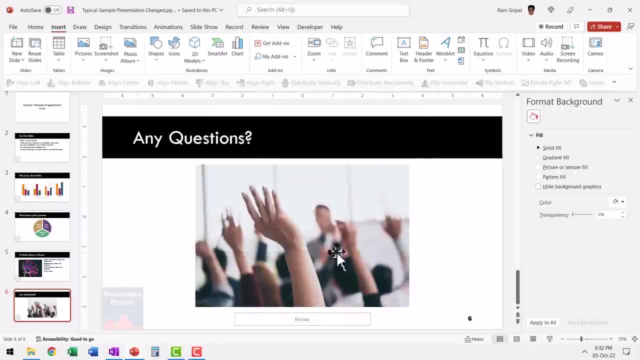 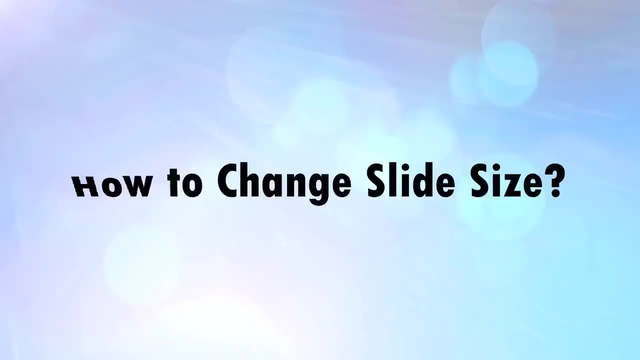 how you add footer to every single slide once again. after doing that, you go to theme slide master and make your corrections here for any of the changes in terms of font size, type, etc. and talking about which theme slide master allows you to change the slide size as well by default. 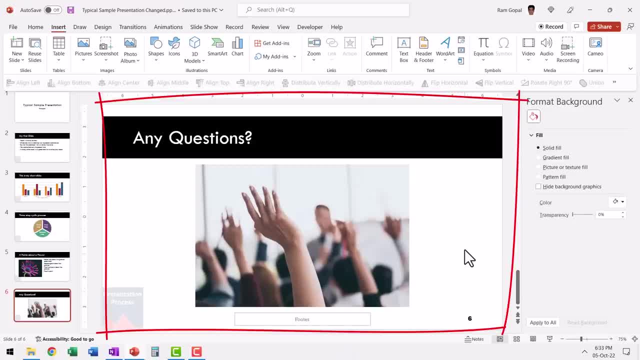 all the latest slides will be in font size and font size will be in font size and font size will be in font size. presentations are made typically in 16 is to 9, which is the wide format. if you want to have the regular standard format of 4 is to 3 ratio, you can do so by going to theme slide master. once again. 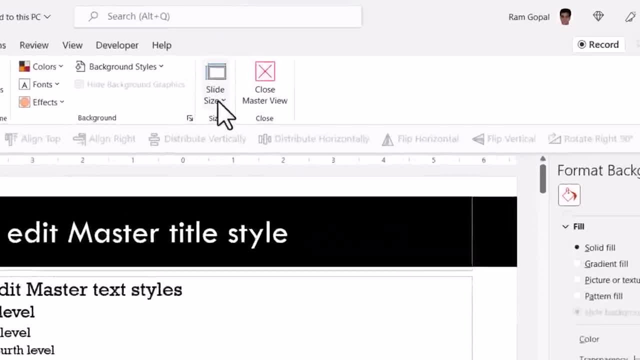 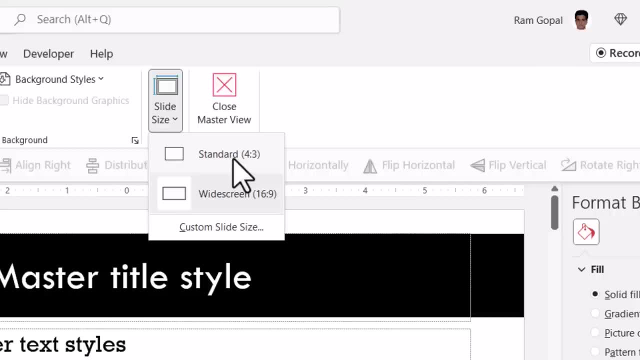 let me go back again to the same thing. go here and you can change the slide size to standard. 4 is to 3, but this is something i would recommend you do right before you create any of your content, otherwise you may have to spend an inordinate amount of time to adjust all the images text boxes. 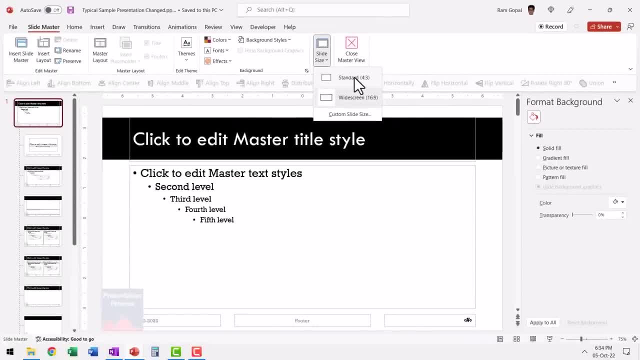 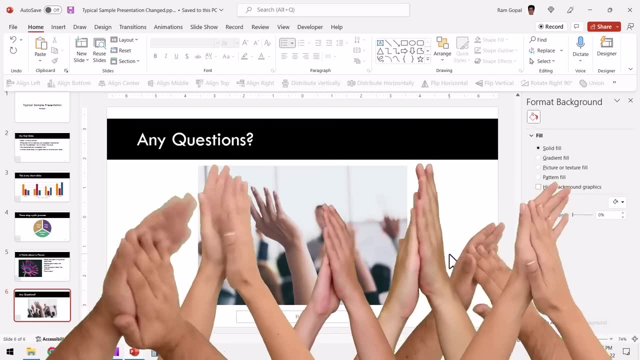 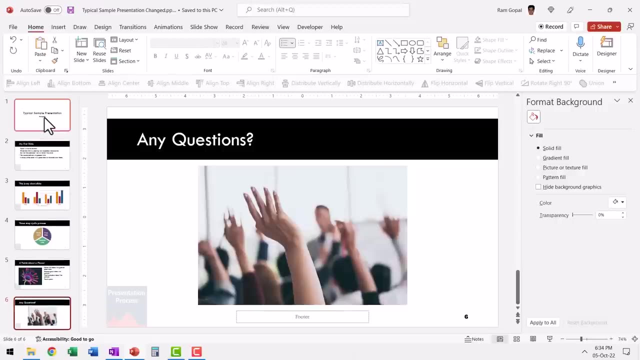 so this is an option you have available right inside theme slide master. now, before we close, i want to give you three additional useful tips that can really impress your audience. one is: you can apply transitions to all your slides quite easily in the theme slide master itself. so let us go here. 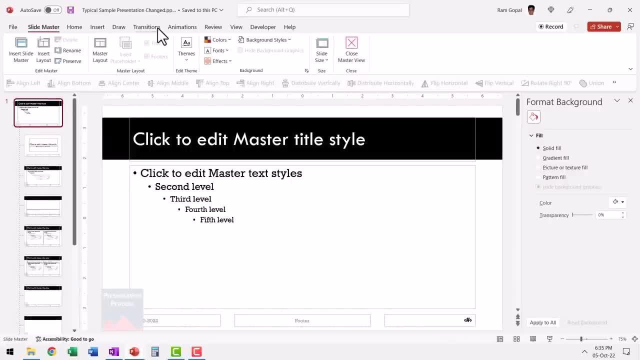 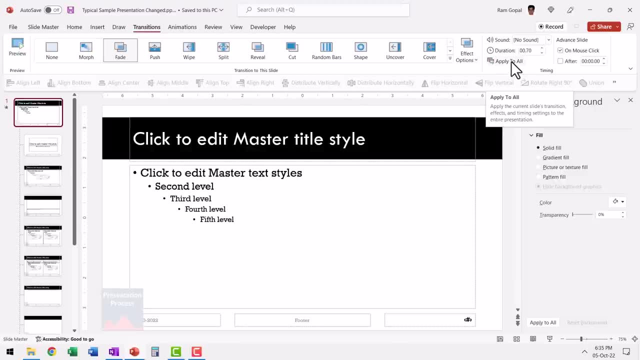 go to shift and then normal view go here and you can go to transitions and you can choose a simple transition, like, say, a fade transition. you can apply to all. of course, you can do that outside of slide master view as well, but then this is another option available for you to apply to your 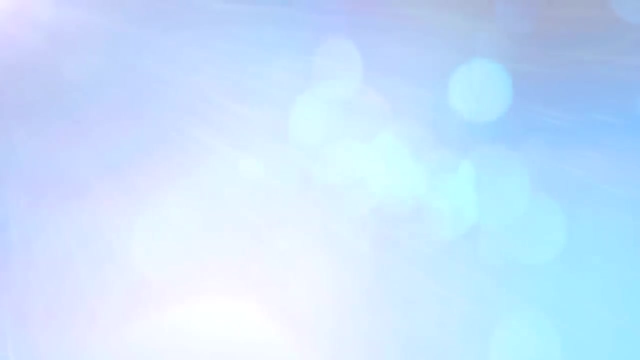 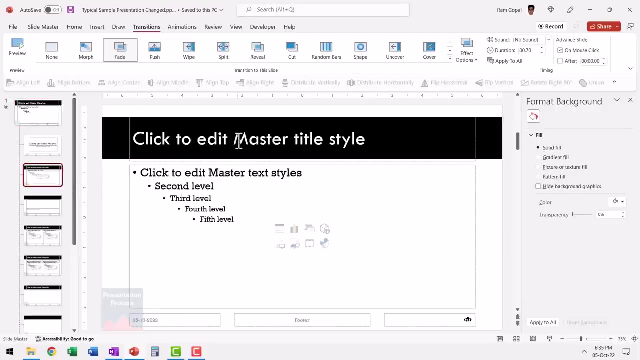 slide master. the next interesting trick is to apply animation to a certain slide layout. for example, let us go to this one, which is the title and content layout, and i want to say that my bullets need to appear with fade animation on click. i can do so by going here and by choosing: 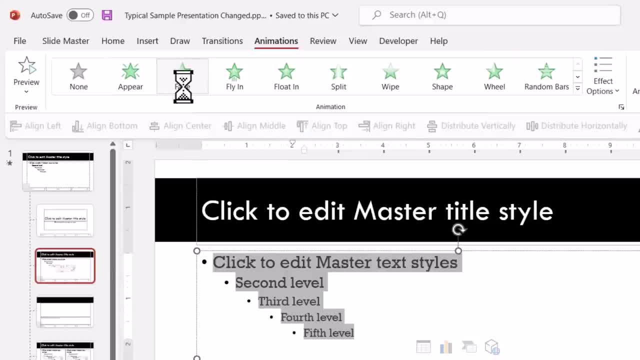 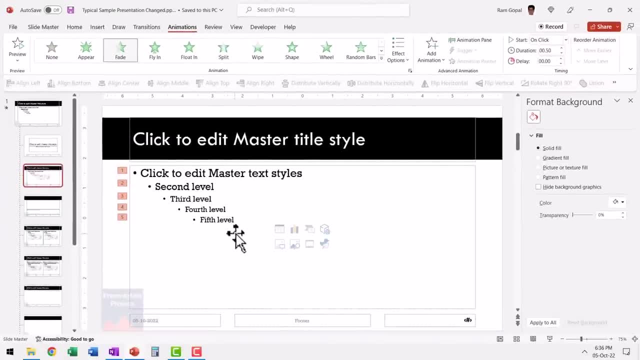 animations. in the animations tab, i can choose fade animation. and i can choose fade animation and say start on click. now every single bullet will come in with a fade animation on click whenever you use this layout as your slide master. now let me take this one step forward. let us go to 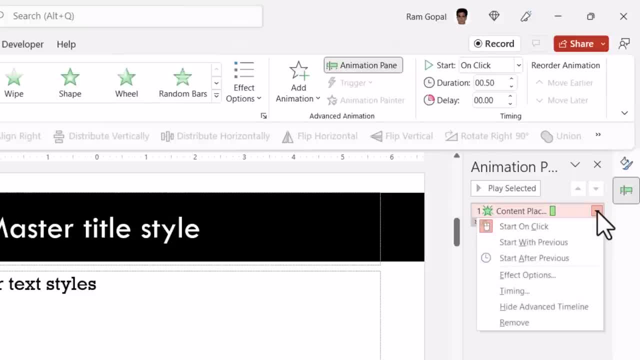 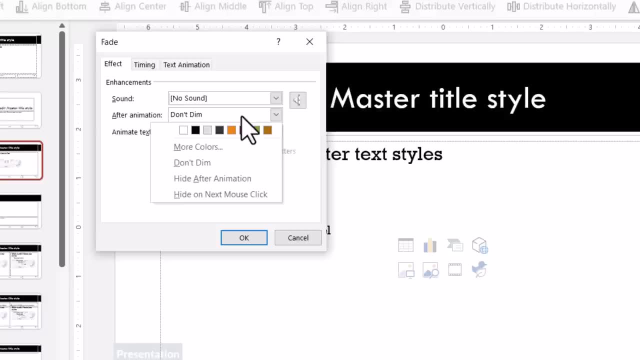 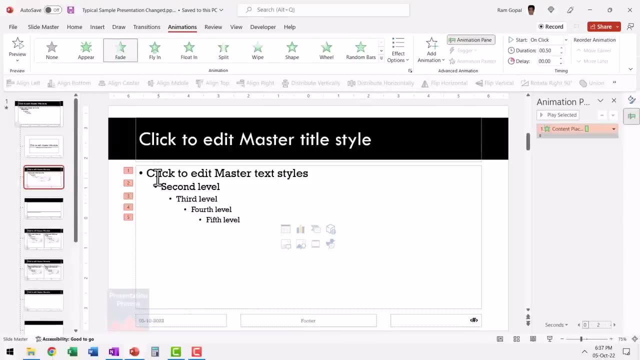 animation pane. here let us open the animation event, go to effect options, and i'm going to do this additional thing, which is, after animation, it should dim into a lighter color like this, and i'm going to say: ok, now the animation is. on a click, the first bullet will appear. then, on a click, the second bullet will. 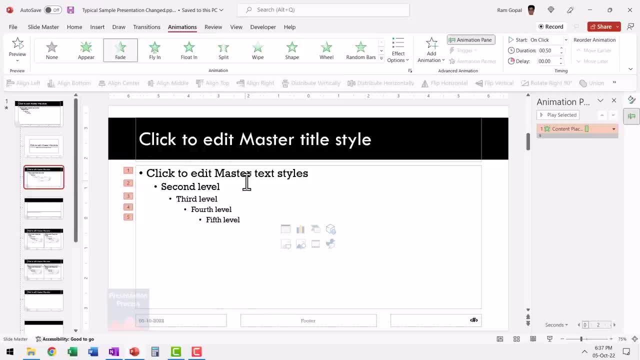 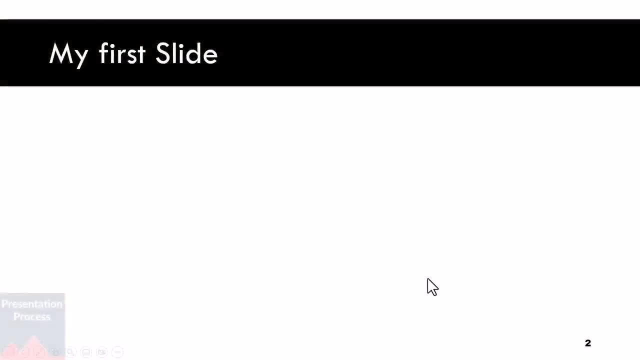 appear, while the first bullet will dim out. let us see how this applies to one of our slides. so let us go to slide master, go to close master view. let us go to slideshow and see how the whole thing works. here you can see that i have not really added any animation. 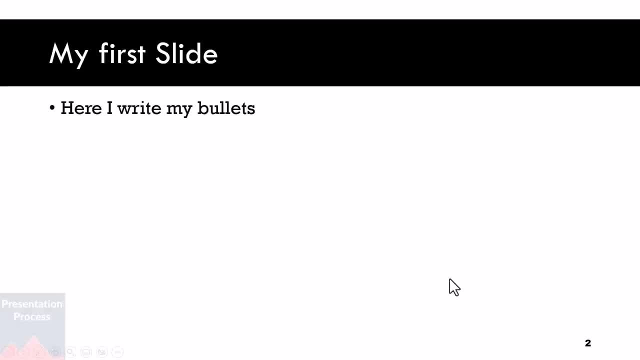 it is part of slide master. on a click i have the first bullet point up here. then on a click you can see that the first bullet dims out and then the next one appears, and then that one also dims out, and it goes on. now let me share the final trick. let us say, you have 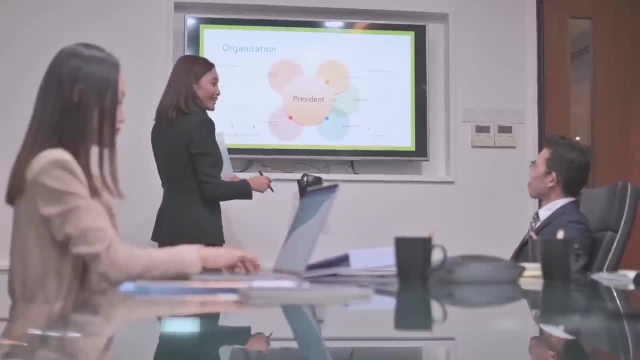 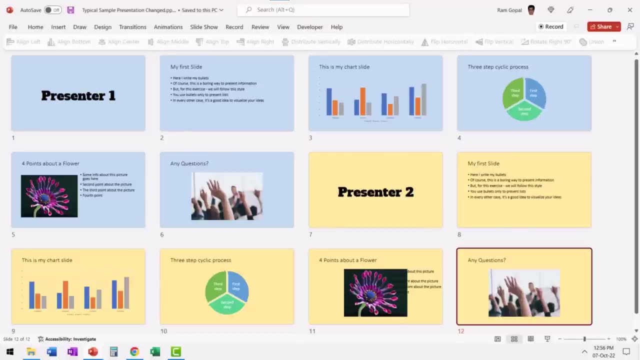 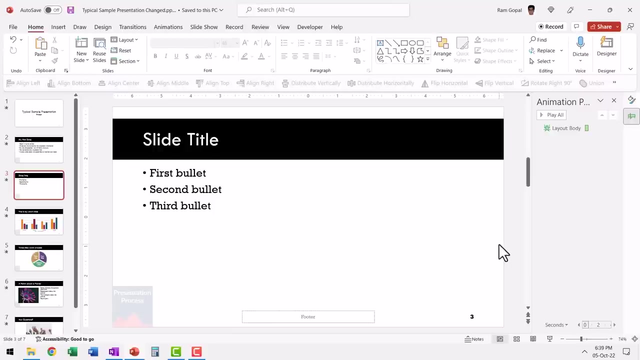 multi-person presentation, that is, two or more people are presenting from the same slide deck. each person presents a different section of the presentation. you can make the different sections visually distinct by having a duplicate of your theme slide master. let me show you what i mean by that. let us go to the theme slide master by holding the shift button. 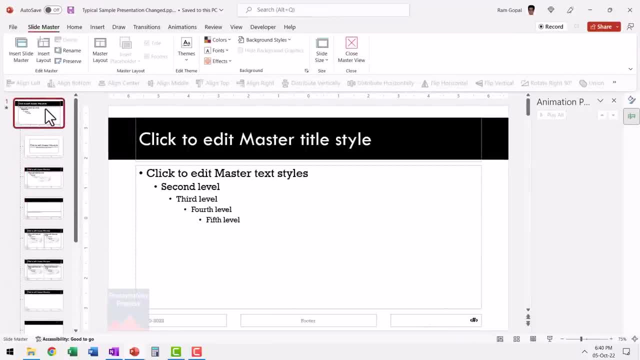 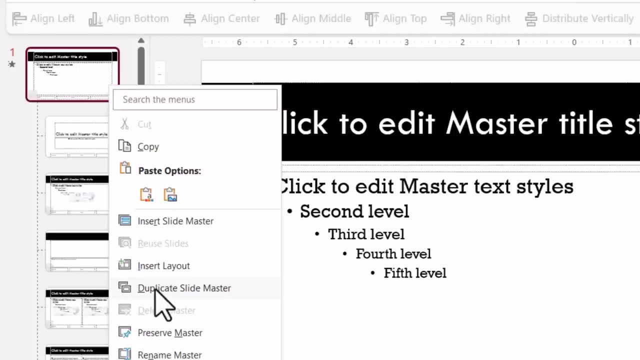 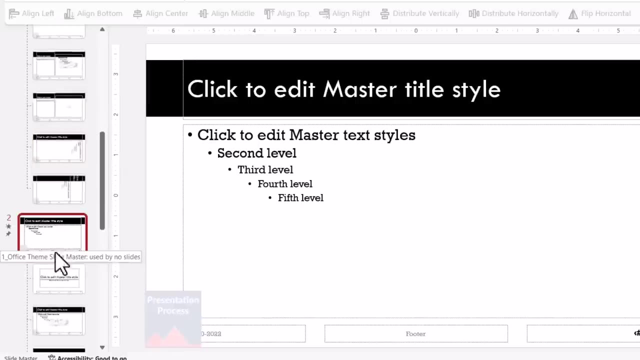 view and you can see that this is one set, one theme slide master and all these child slide layouts. now i can right click and go to duplicate slide master option. you can see that the first one is duplicated and now we have a new theme slide master and the corresponding layouts. 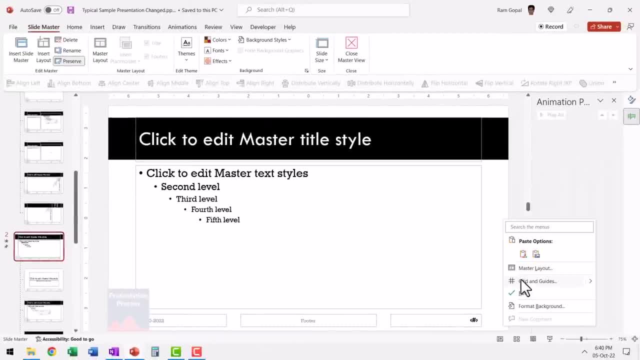 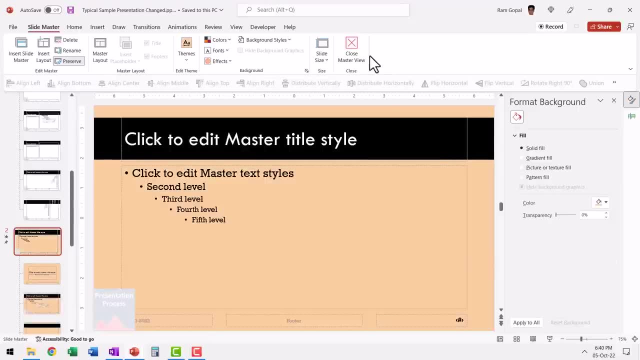 here i can add a different background, so let me right click, go to format background and let us give this a very light, maybe this kind of orange accent color, and let me close master view now. at this point you may not really see any of the slides in that particular. 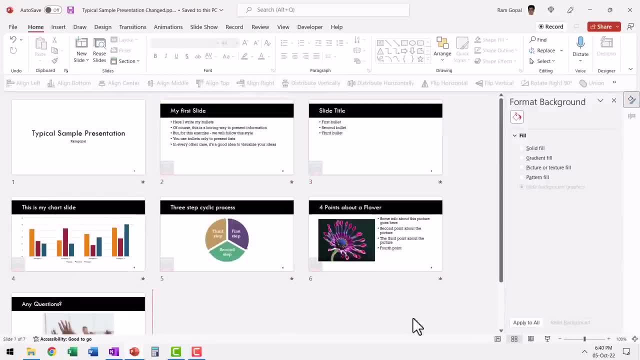 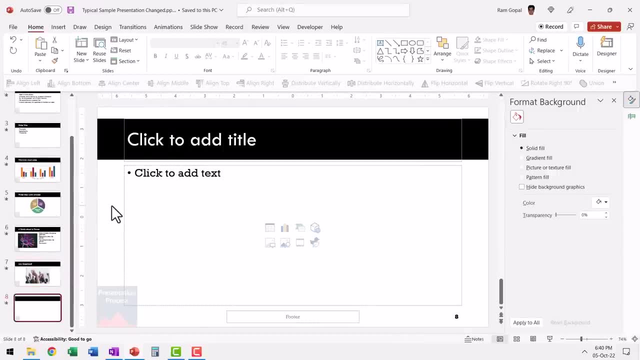 color. but if i were to introduce a new slide, let me go to the normal view. let us add one more slide here. let us assume that this is a new section and for this i want to choose a different layout. so let us right click, go to layout, and the layout i would want to choose is this one you can see. 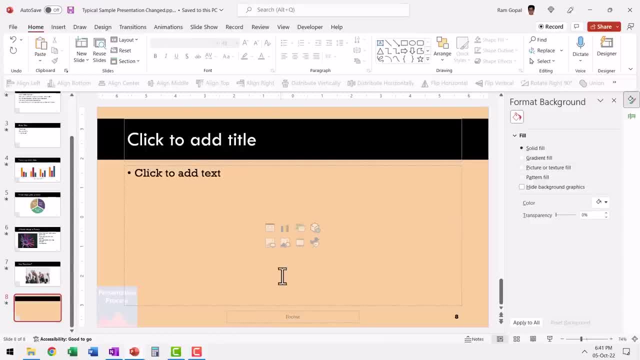 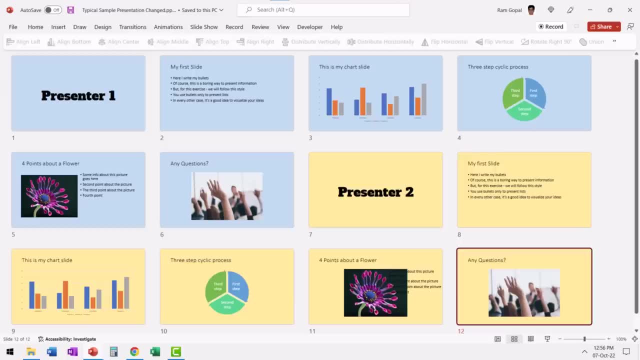 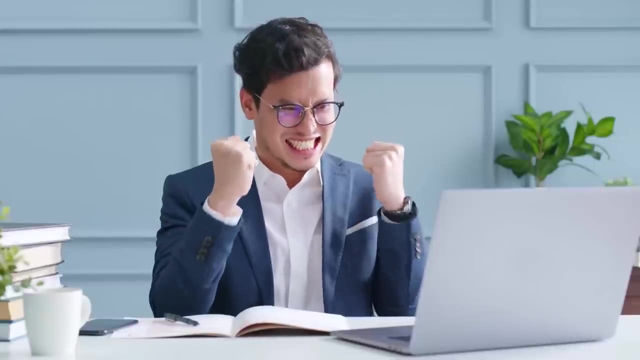 that my new section can have this color. so now when i go to slide sort of view, i can visually distinguish different sections because of their different color background, and it makes it easier for different people to present their sections. now, before we go, one final bonus tip, and that is: 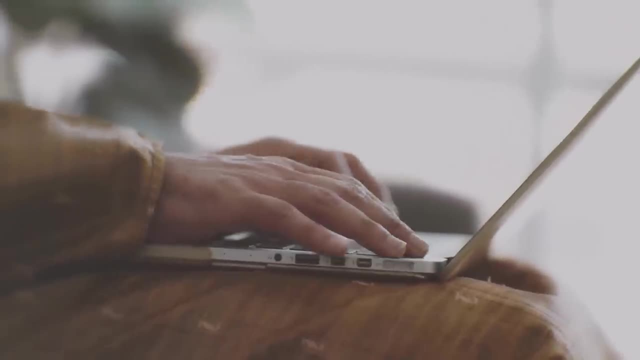 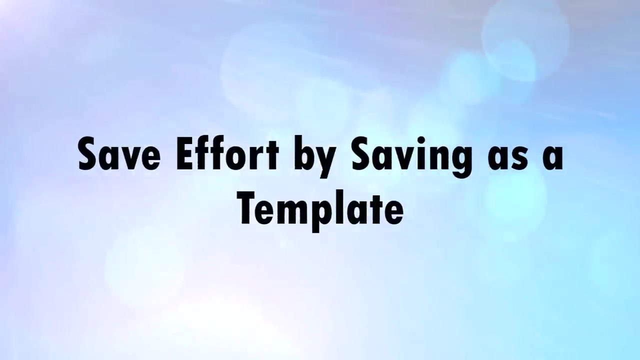 if you want to reuse all the hard work that you had put in in designing one presentation, you can save the presentation as a template. so the next time you want to start a new presentation, you can start the presentation from this template. so all the changes that you had made in the slide master. 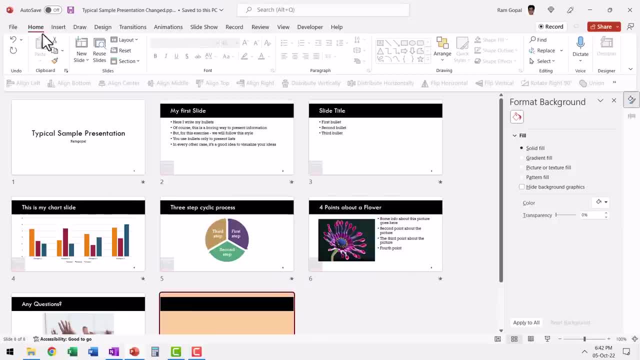 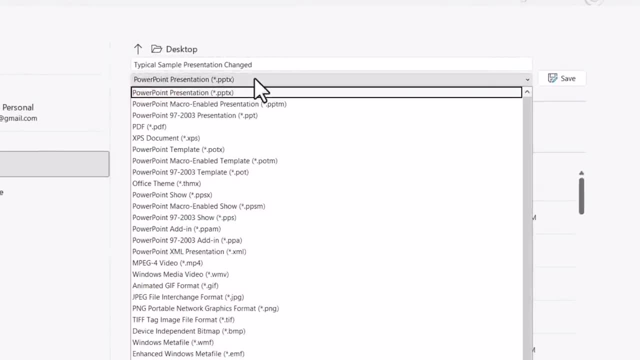 will reflect in the new presentation as well. how do you do that? let us go to file save as, and here i want to change the save type as a template. let me go down here. we have this option called powerpoint template. star dot potx. you can. 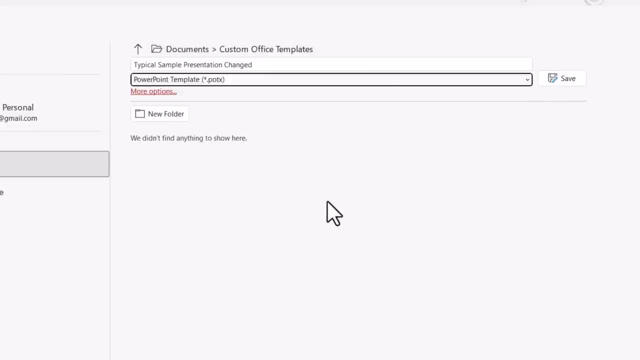 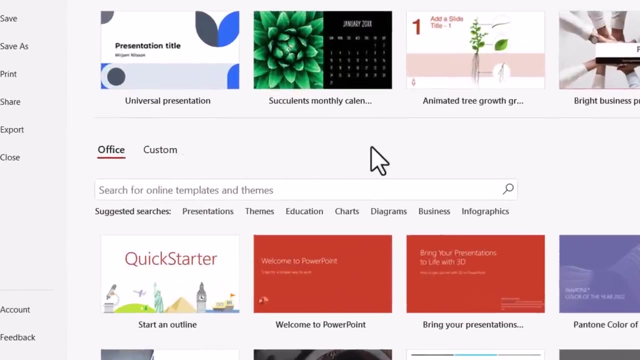 select that and you need to save now. i would highly recommend that you don't change the place where your templates are stored. just go with the flow and you say save now. let me start a new presentation. let me go to file new. this time i want to choose a custom template, so let us go to custom. 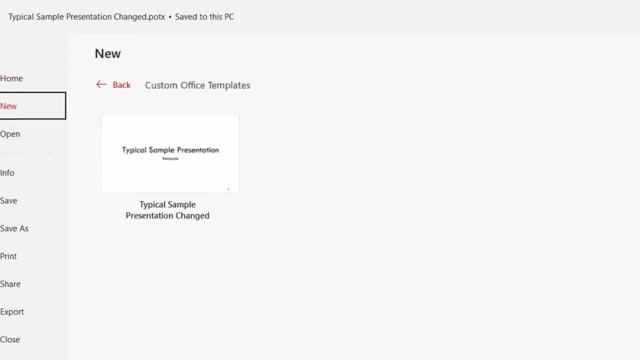 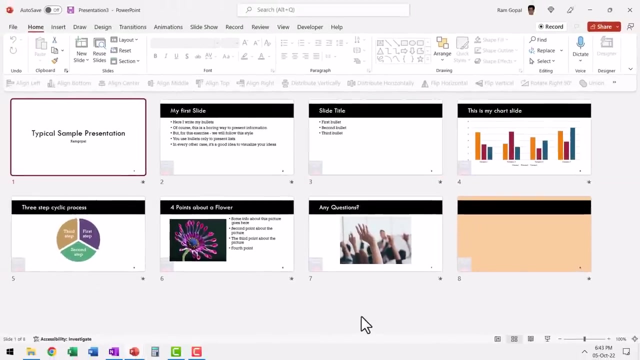 and here i have custom office templates. let me double click and here i have the new template that i had created, which is typical sample presentation, changed. i can click and i'd be able to create a new presentation. by clicking on create option, a new presentation is created.